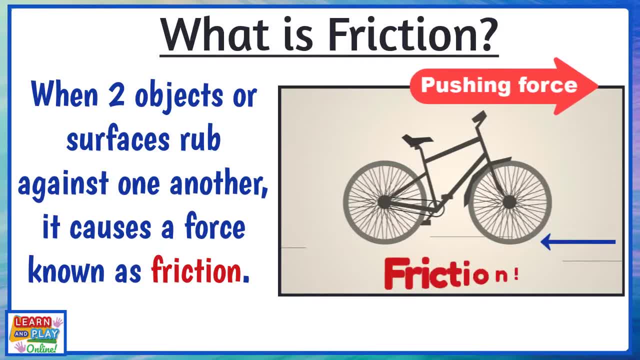 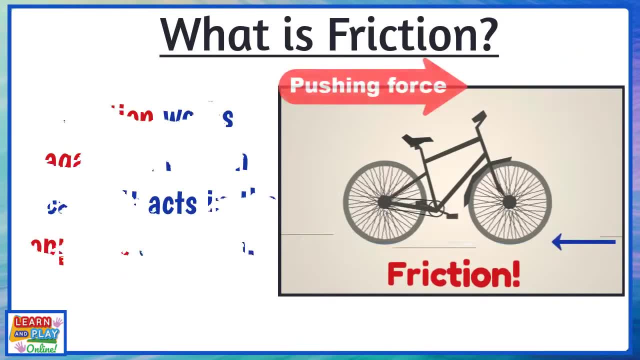 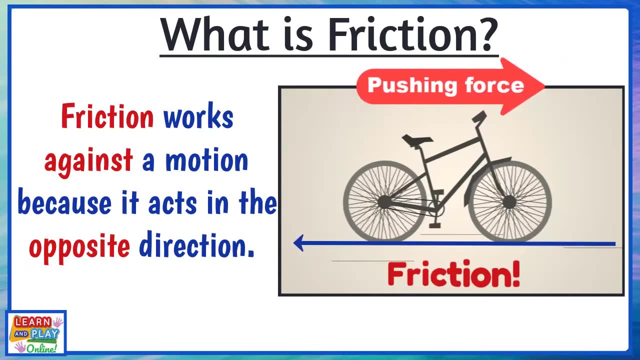 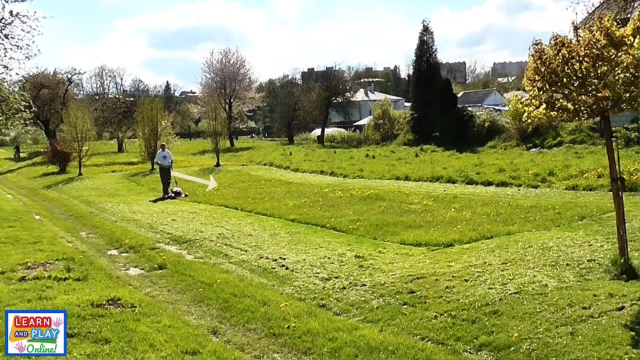 are rubbing against the surface of the ground. Friction is the resistance force that is pushing in the opposite direction of the wheels of the bike. Friction works against a motion because it acts in the opposite direction. Let's look at another example. This man is pushing the lawn mower forward to cut the grass. The lawn mower is moving. 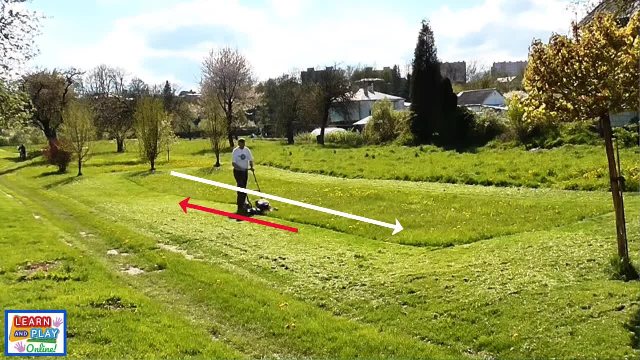 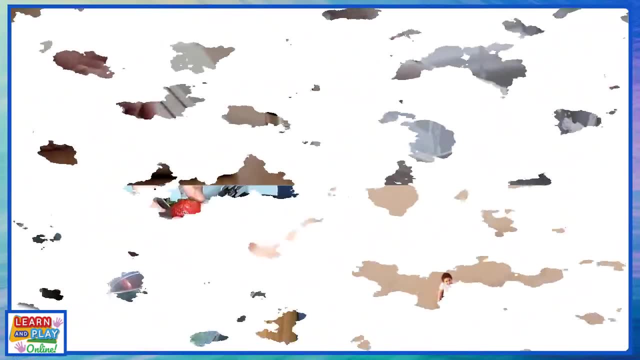 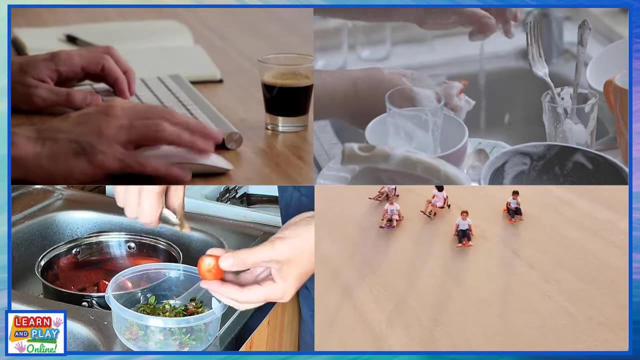 against the surface on the ground. As the lawn mower is pushed forward, it met by frictional forces on the ground. Friction is a part of our lives on a daily basis. Without friction we wouldn't be able to perform simple everyday activities because everything would continue to slide as there. 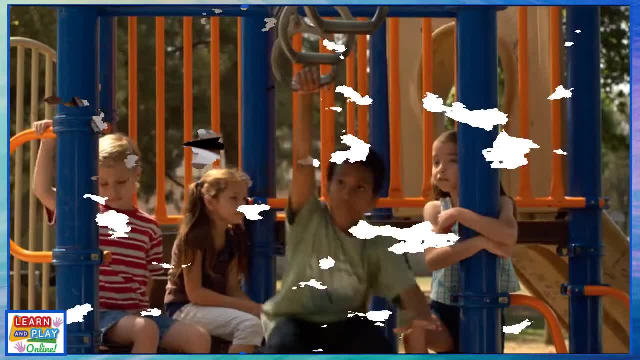 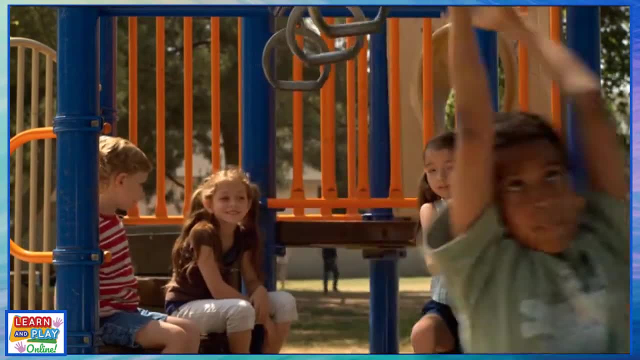 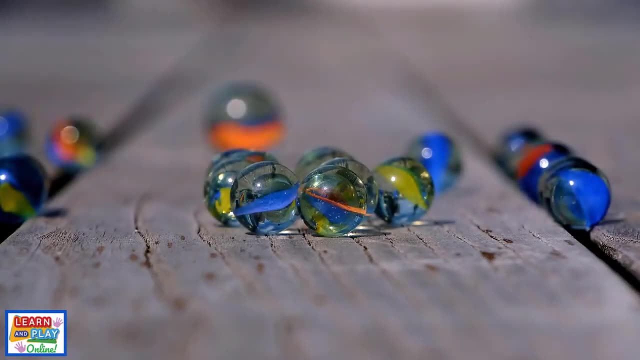 is no force to stop it or slow it down. Thanks for watching as friction would. we need friction because it allows us to grip, hold and move objects in the direction we need or want them to be moved. the amount of friction between objects and surfaces is dependent on things such as how smooth or rough the surface is and how light or heavy the 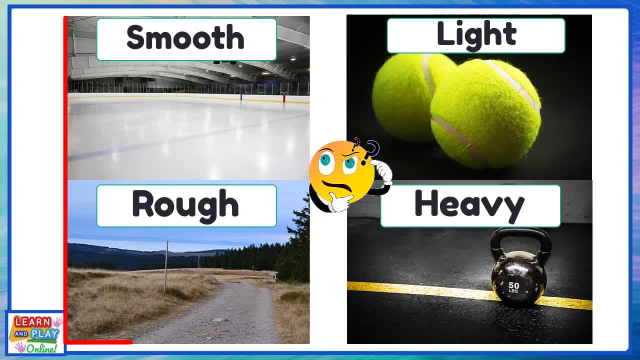 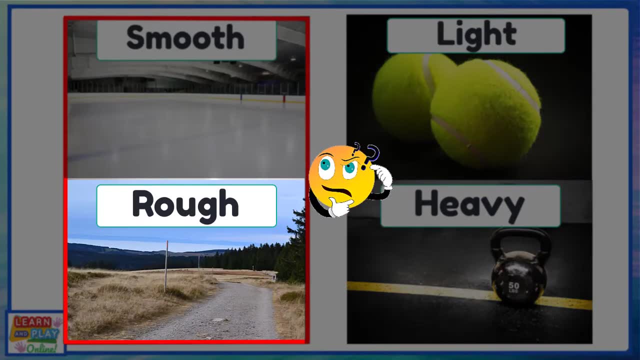 object is. let's think about the smooth and rough surfaces here. if you wanted to go ice skating, which surface would give you less friction so that you can glide smoothly? a surface that's as smooth as an ice rink, or a concreted area that has a rougher surface? well, of course, skating on an 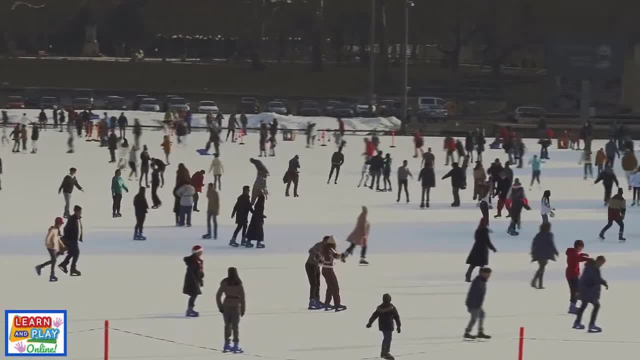 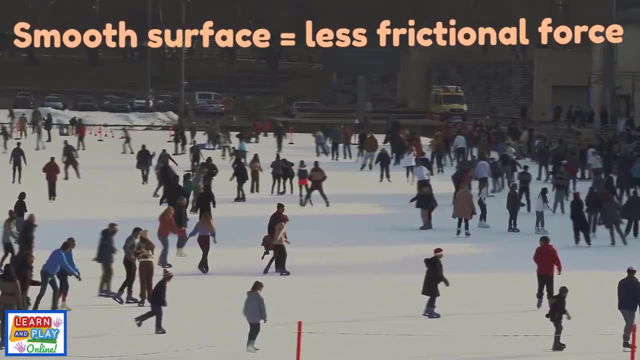 ice rink would give you the best experience. this is because the blades on your ice skates would be rubbing against the smooth surface of an ice rink, which means there is less friction, and that allows you to skate more freely, as there is less frictional force. 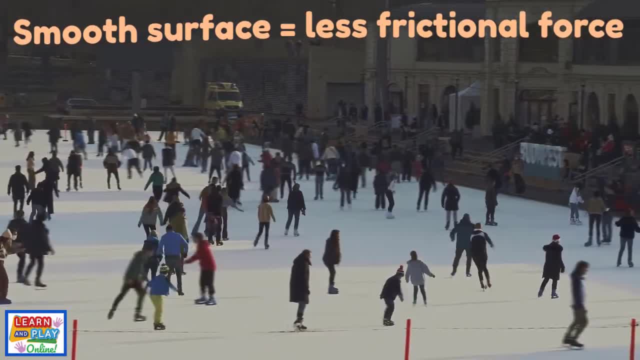 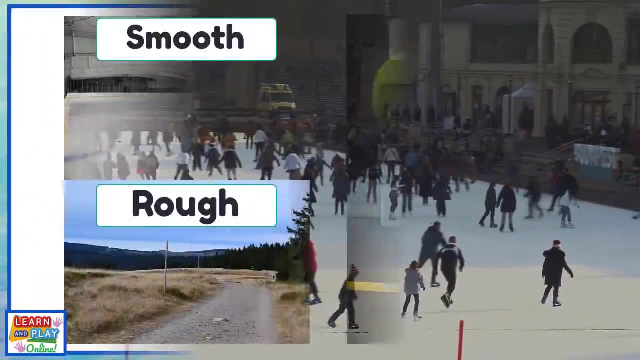 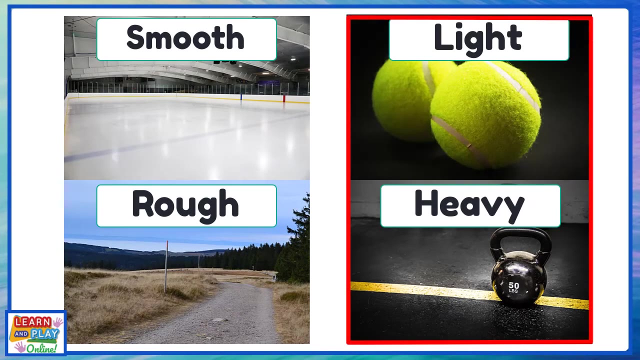 going in the opposite direction. you would definitely not be able to skate like this on a rough surface, as there would be too much friction. now let's think about how the amount of friction would be affected, depending on the weight of an object. the heavier the object is.